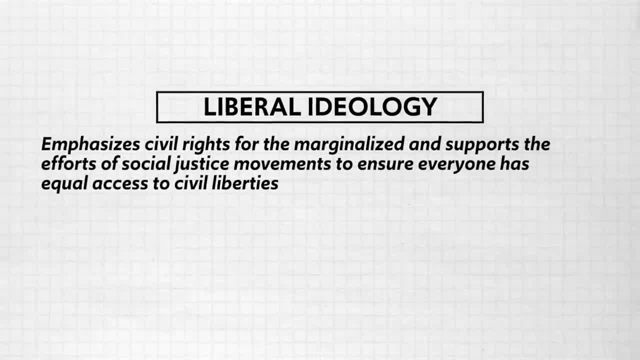 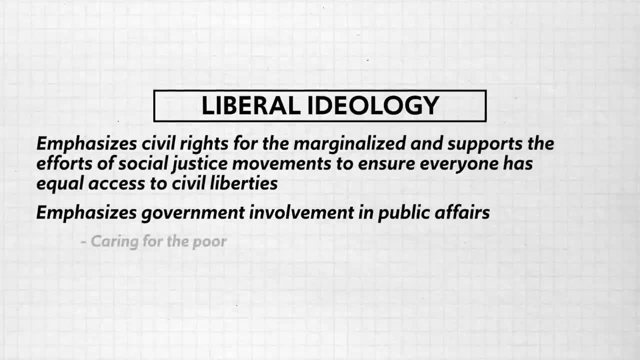 emphasize civil rights for the marginalized and supports the efforts of social justice movements to ensure that everyone has equal access to civil liberties. Additionally, liberals tend to emphasize government involvement in public affairs, which would include care for the poor and regulations on businesses and intervention in the economy. Or to say it another way, liberals look at what exists and says: 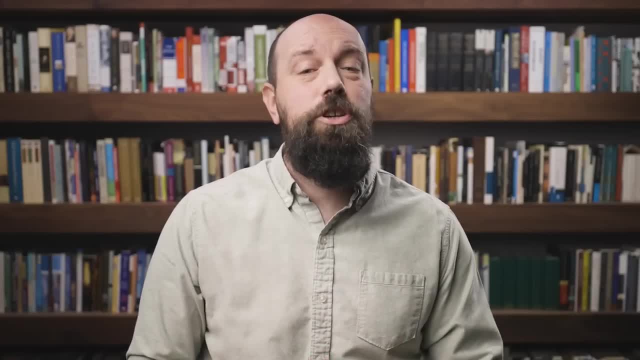 uh, it is broke, so let's fix it Now. there's a third ideology you should know, namely libertarian ideology, but we're going to look at that in another video For our purposes. here we're just sticking to conservative and liberal ideology. 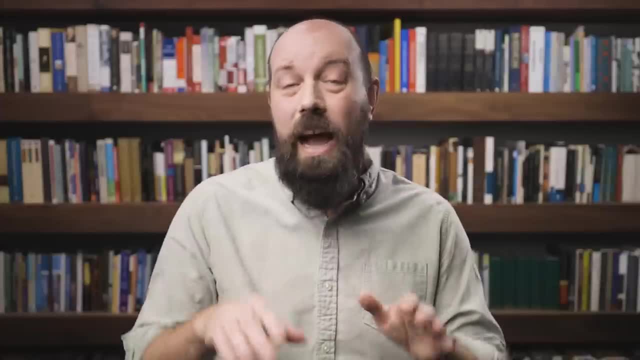 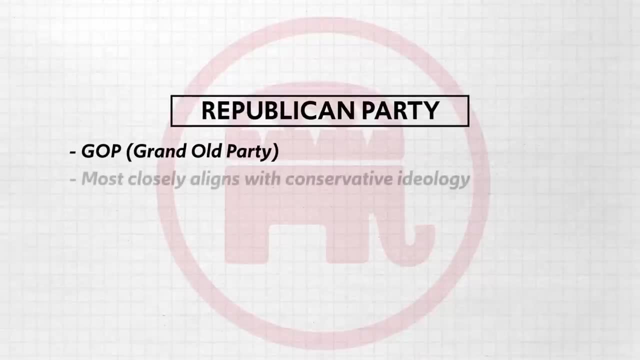 Okay, let's turn the corner and talk about the two major political parties in America and how they align with the ideologies we just talked about. The Republican Party, often referred to as the GOP or the Grand Old Party, most closely aligns with conservative ideology, And the way that you know that is by looking at. 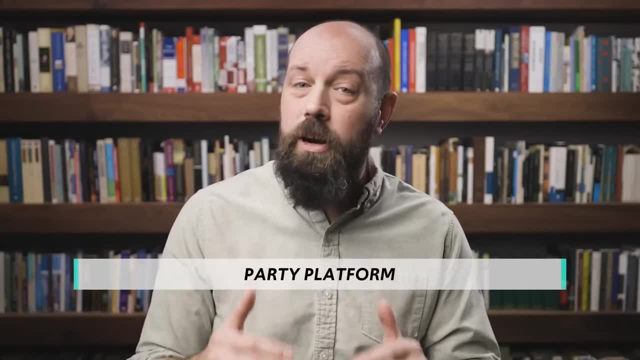 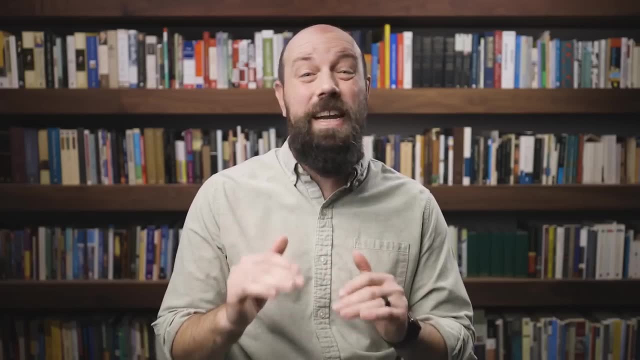 their party platform, which is a set of policy goals published by the party, which tells you the kinds of legislation they would pursue should their candidate win an election. So if you look at the Republican platform you can see conservative ideology dang near everywhere. Here in the section on the economy they say: 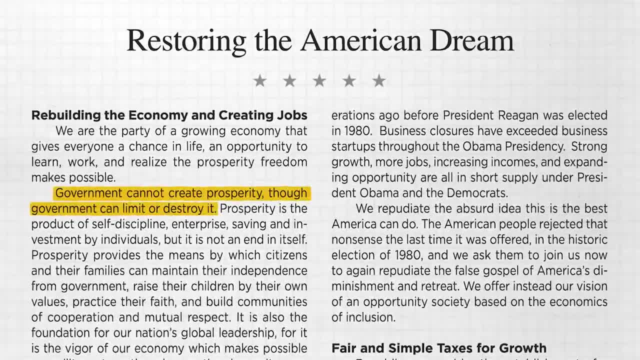 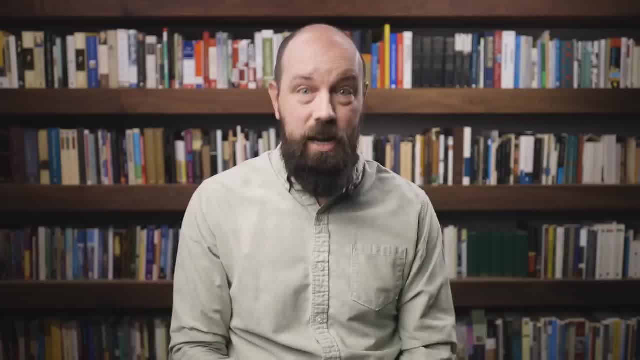 government cannot create prosperity, though government can limit or destroy it, And that is a conservative ideology The Republicans believe. get the government out of the economy, deregulate businesses and let the free market take care of the economy. In the section on what a constitutional government should look like, they say this about the family: 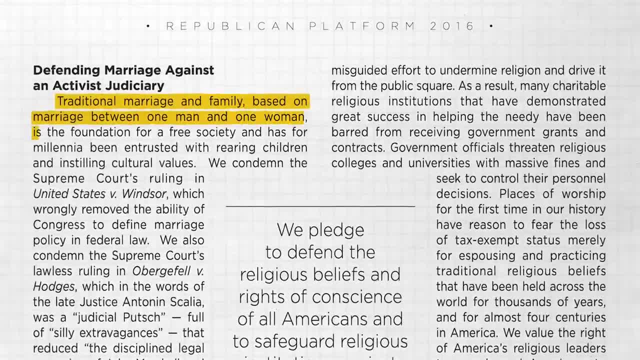 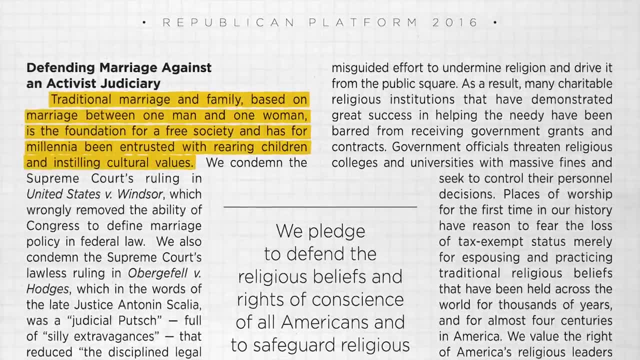 Traditional marriage and family based on marriage between one man and one woman is the foundation for a free society and has for millennia been entrusted with rearing children and instilling cultural values. So again there you have: conservative ideology reaching backwards to establish traditions and seeking to uphold them. If it ain't broke, don't fix it. Additionally, the Republicans, when it comes to social programs, style themselves as the party of personal responsibility, So it's no surprise to see that reflected in their platform in the section about social welfare programs. 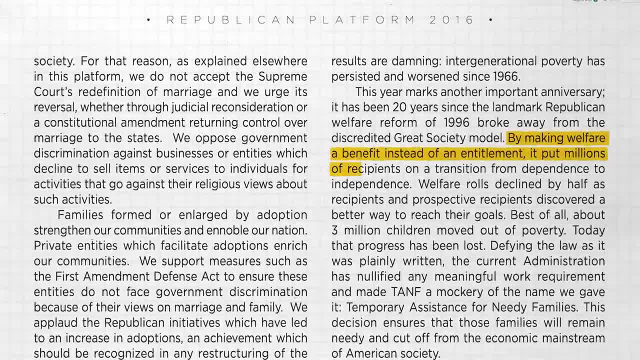 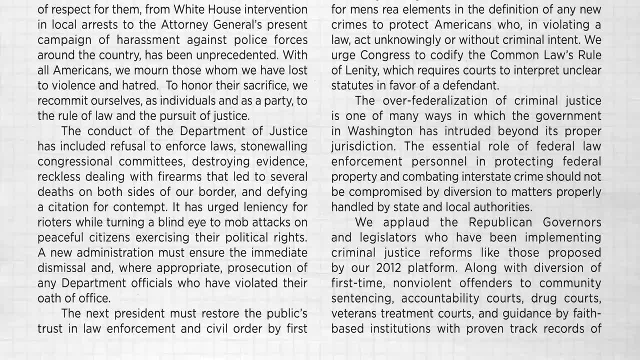 By making welfare a benefit instead of an entitlement. our policies put millions of recipients on a transition from dependence to independence, And the Republicans also regard themselves as tough on crime. For example, they say To honor the sacrifice of police officers, we recommit ourselves as individuals and as a 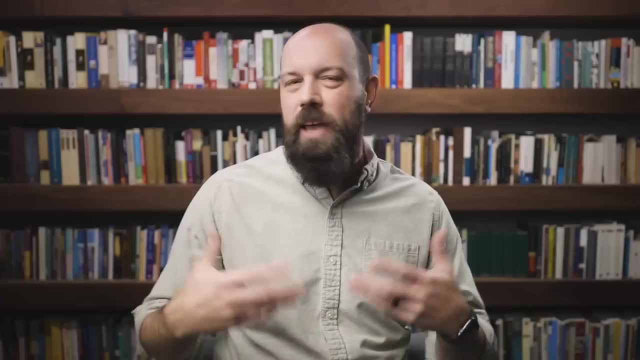 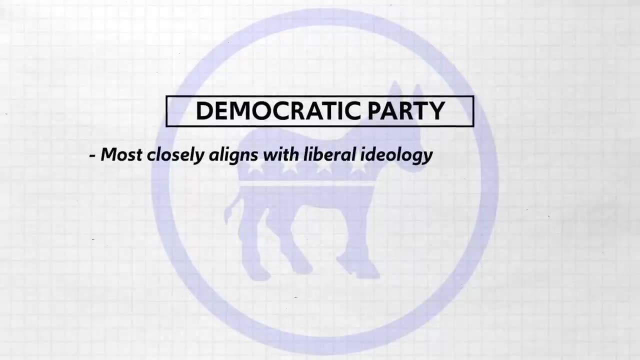 party to the rule of law and the pursuit of justice. So I only gave you a sample of the platform, but you can see that Republicans generally hold to conservative ideology. Now let's have a look at some of the examples of liberal ideology in the platform of the.